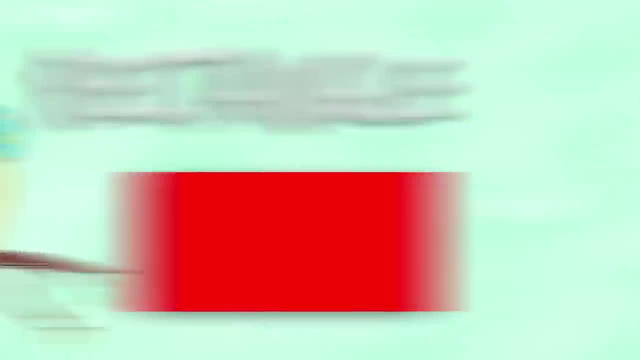 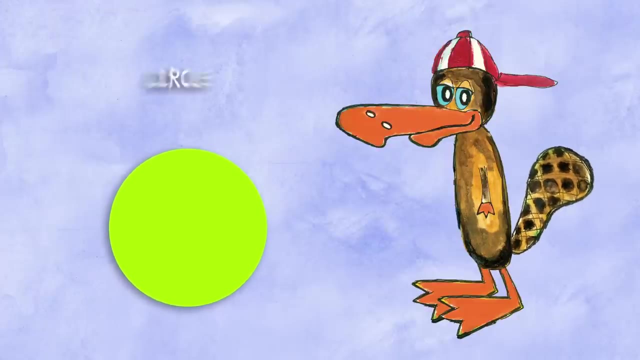 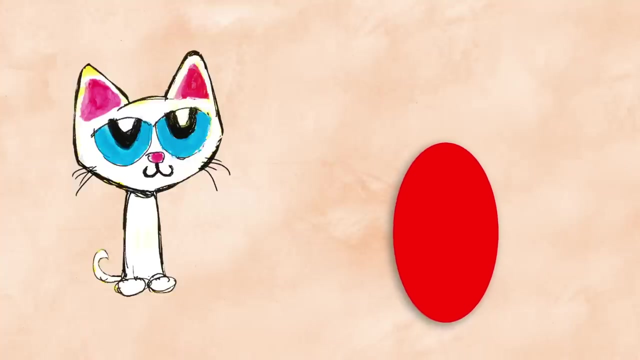 That's a rectangle. Wow, Wait, this shape is perfectly round. What could that be? Oh, it's a circle. So cool, This looks like a circle, but it's all smushed. Hmm. Oh yeah, that's called an oval. 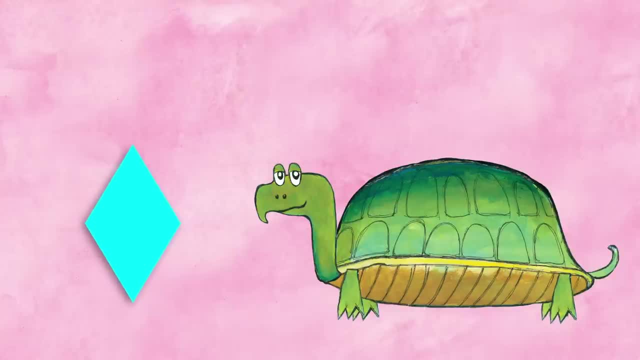 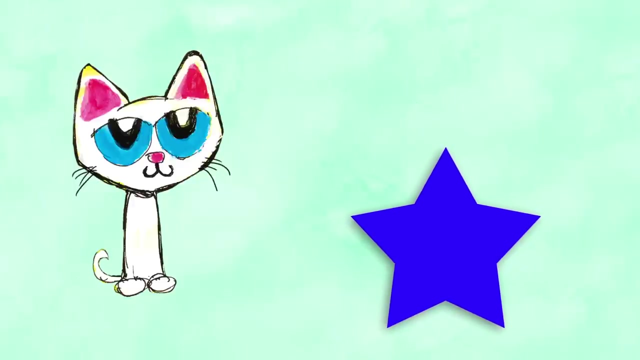 Groovy. Here's one that has four sides like a square, but it stands on a point. What do we call that? It's a diamond. Out of sight, This shape looks like five triangles put together. What's that called? It's a star. 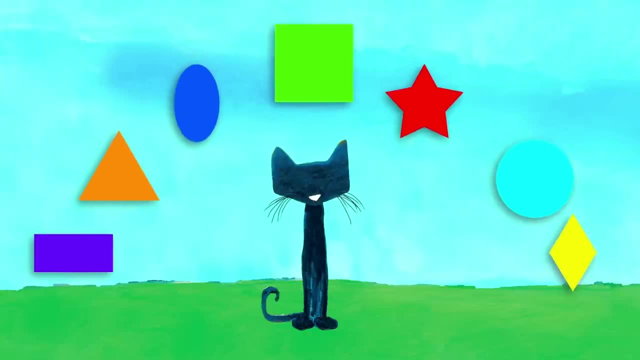 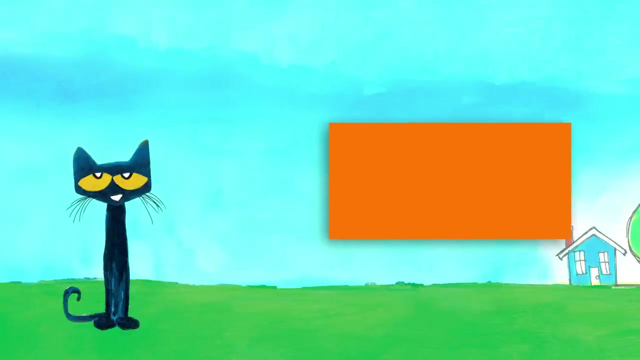 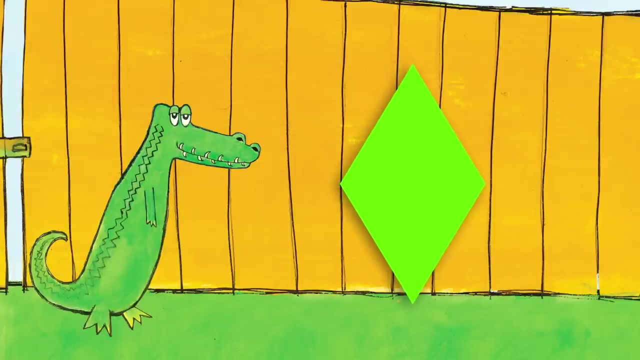 Wow, Those are the basic shapes, And now that you've seen them, let's look again. Ready, Let's do it. Square- Rectangle- Diamond Triangle Circle. Oval Star Square- Rectangle- Diamond Triangle Circle. 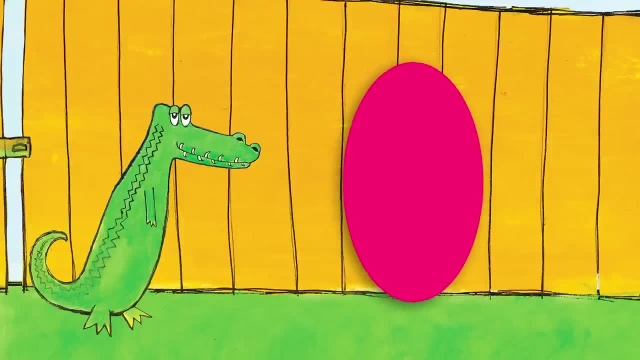 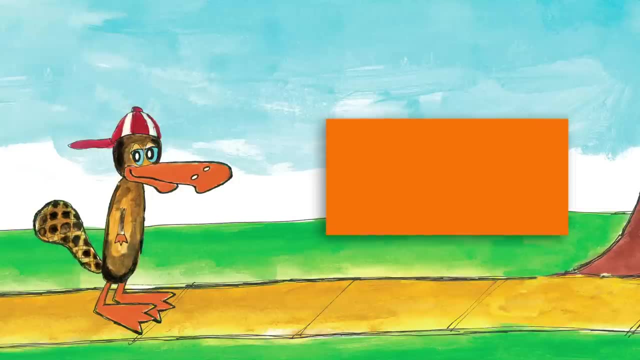 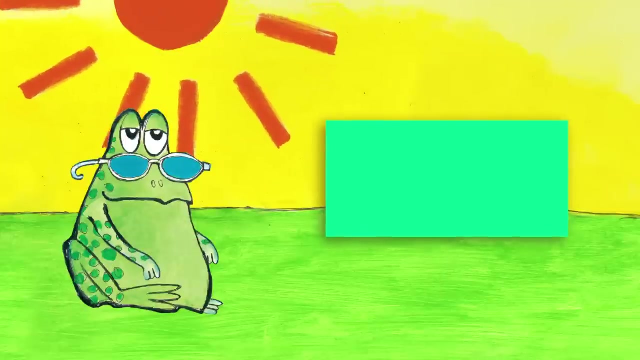 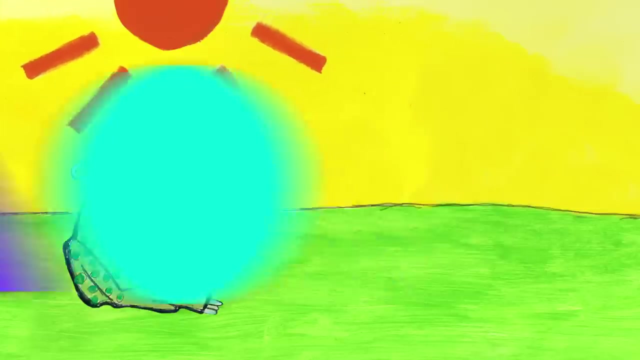 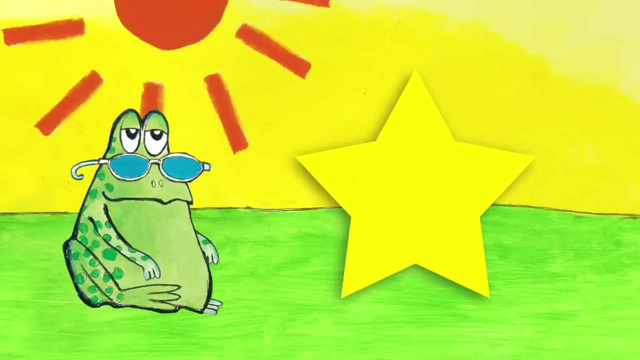 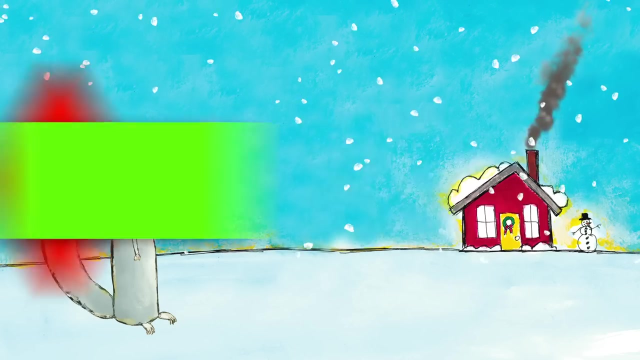 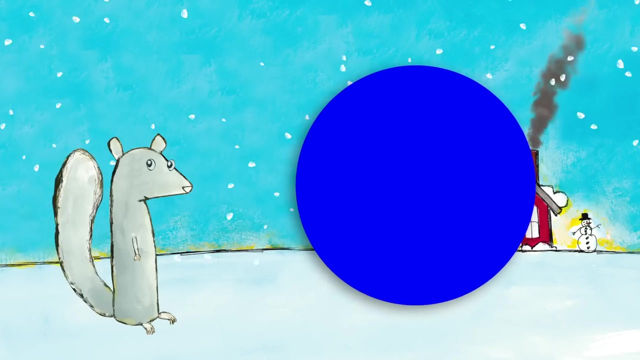 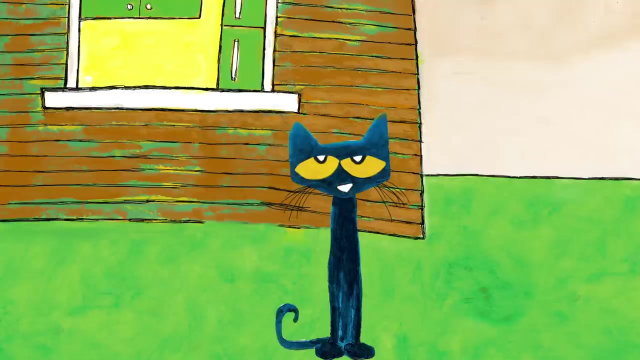 Oval Star Square. Rectangle Diamond Triangle Circle. Rectangle Oval Star Square. Rectangle Rectangle Diamond Triangle Circle. Oval Star Square. Rectangle Diamond Triangle Circle, Oval Star. Super cool, You're doing such a great job. Wanna try it a different way. 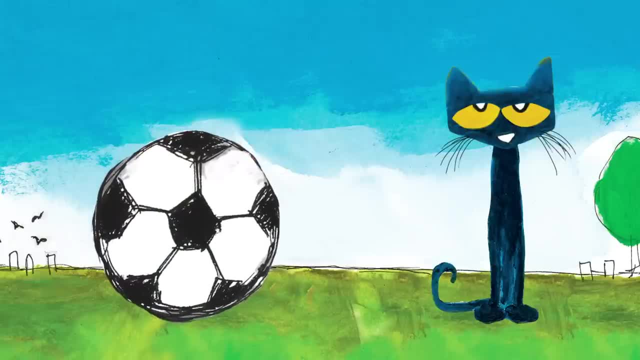 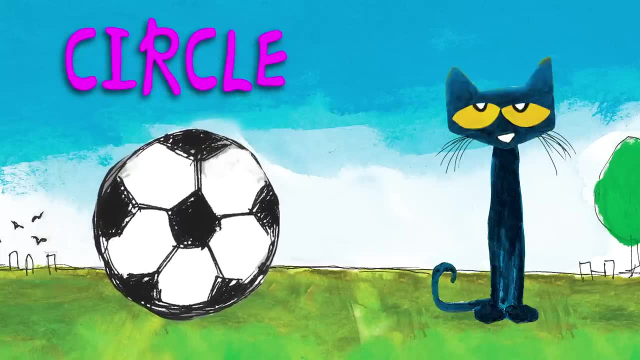 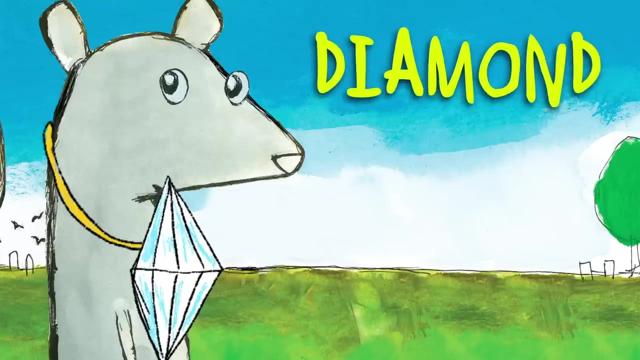 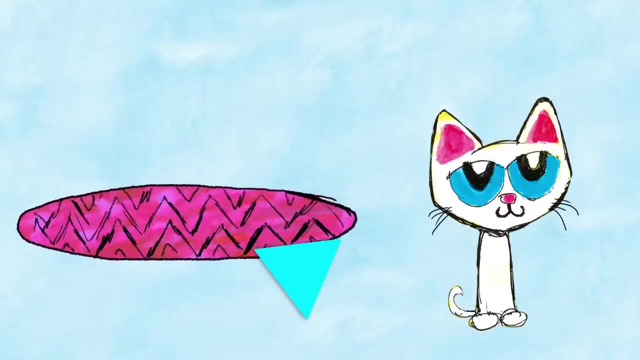 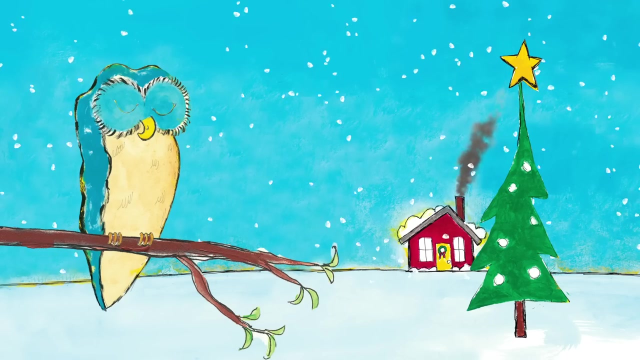 Let's go. What shape is Pete's soccer ball Circle? What shape is Squirrel's necklace Diamond? What shape is the fin on Callie's surfboard Triangle? What shape is the top of Owl's Christmas tree Star? What shape is Turtle's house? 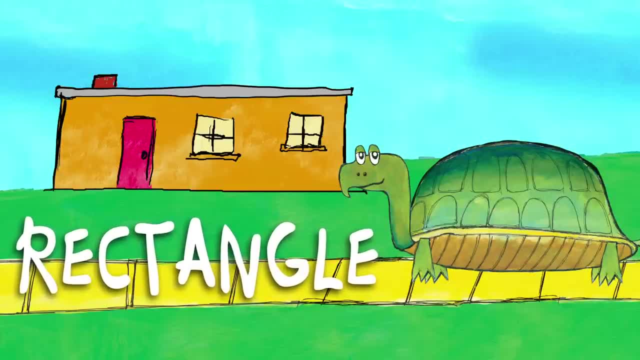 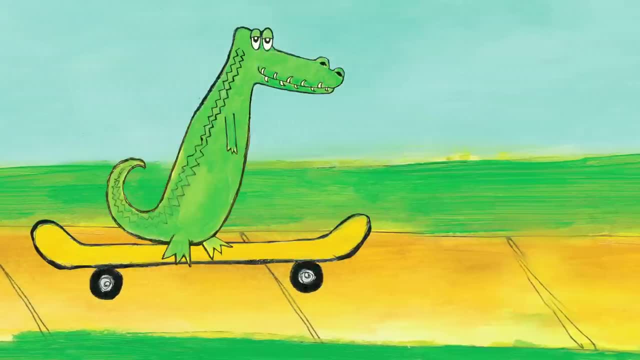 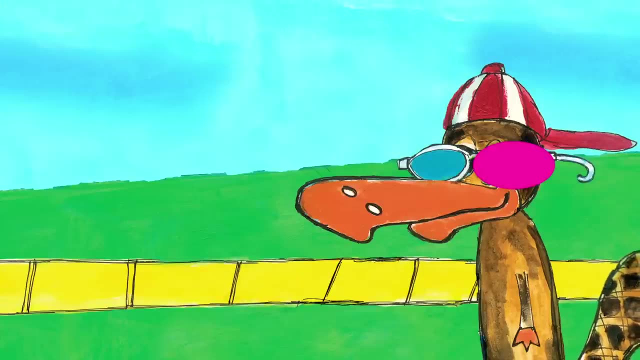 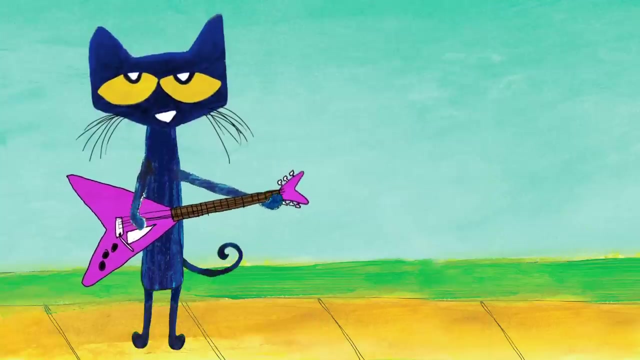 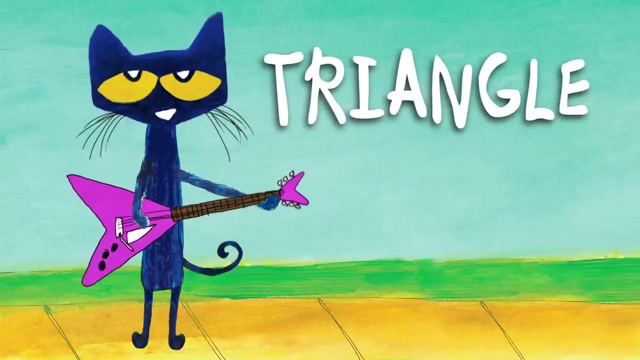 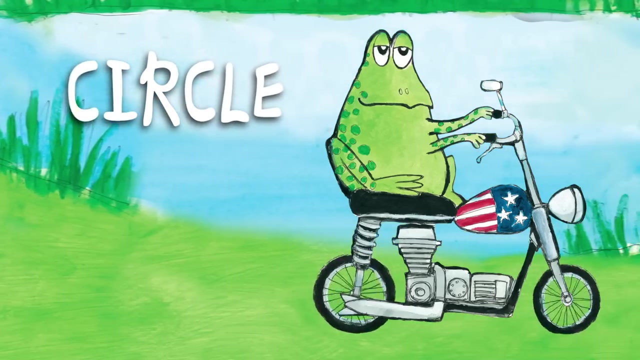 Rectangle Triangle. What shape are the wheels on Alligator's skateboards Circle? What shape are Gus' sunglasses Ovals. What shape is Pete's guitar- Triangle Triangle. What shape is Grumpy Toad's motorcycle wheel Circle? What shape is the decoration on Callie's cupcake? 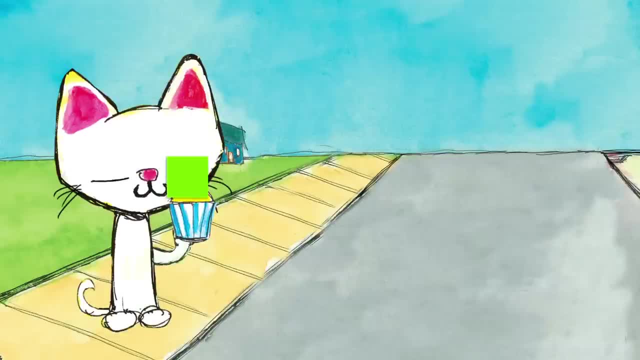 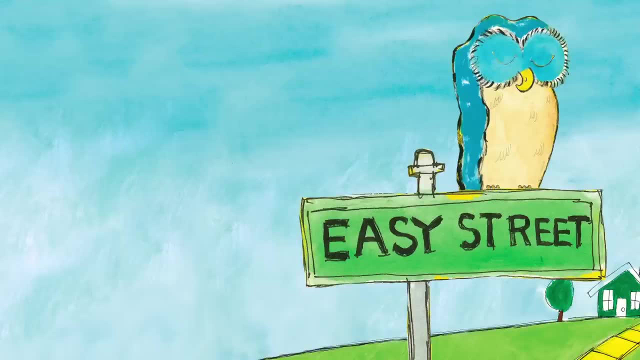 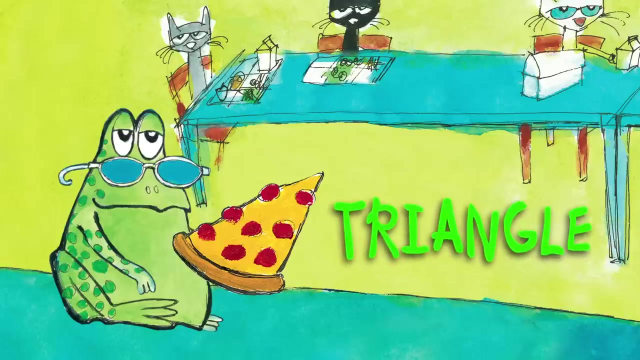 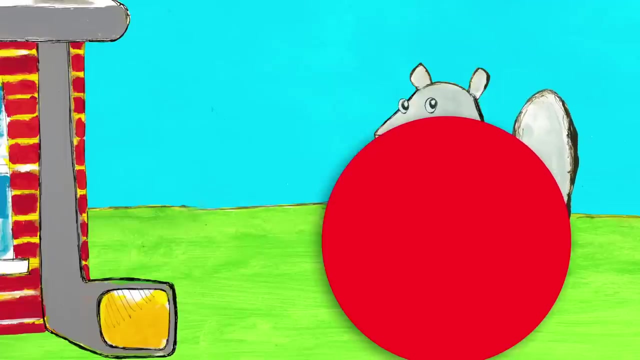 Square. What shape is the sign on Owl's street, Rectangle Triangle Square? What shape is the sign on Owl's street, Rectangle Triangle? What shape is Grumpy Toad's slice of pizza Triangle? What shape is Squirrel's tambourine Circle? What shape is Callie's pumpkin? 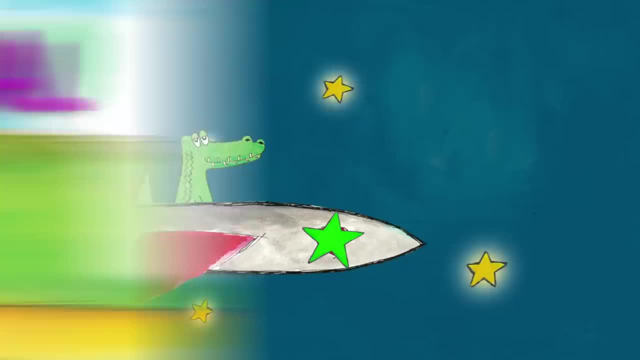 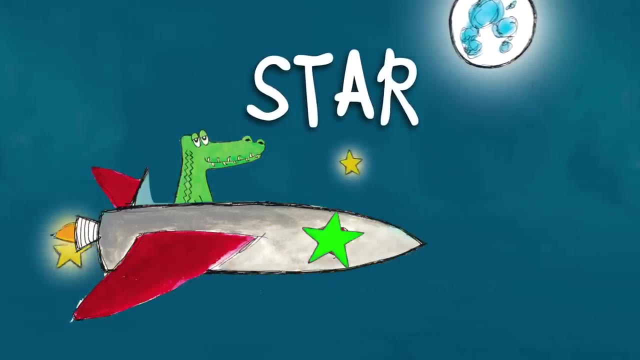 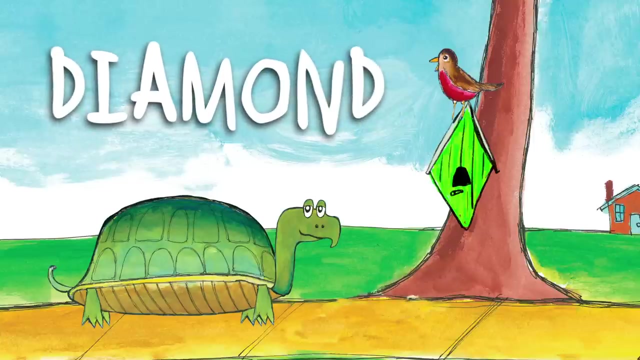 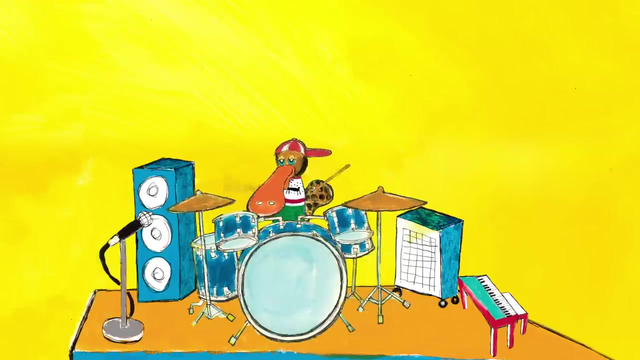 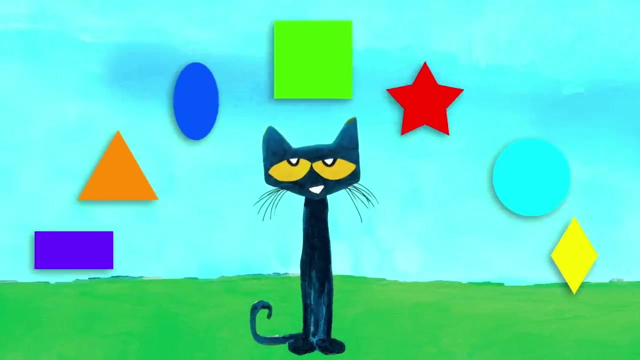 Oval. What's the shape painted on Alligator's rocket ship Star? What shape is Turtle's bird feeder Diamond? What shape is Gus's bass drum Circle? Great job, I think you understand what shapes are now. Wow, That was so groovy. 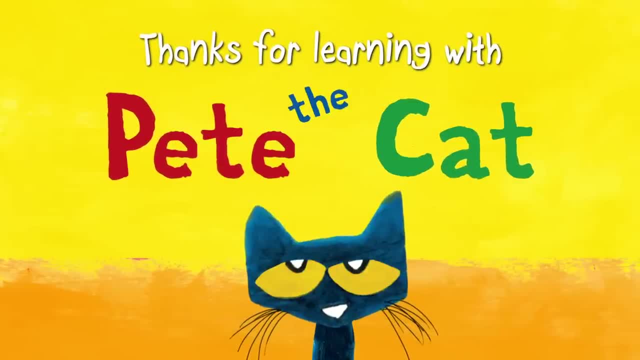 Thank you, Thanks for learning with Pete the Cat. See you next time. Bye-bye.